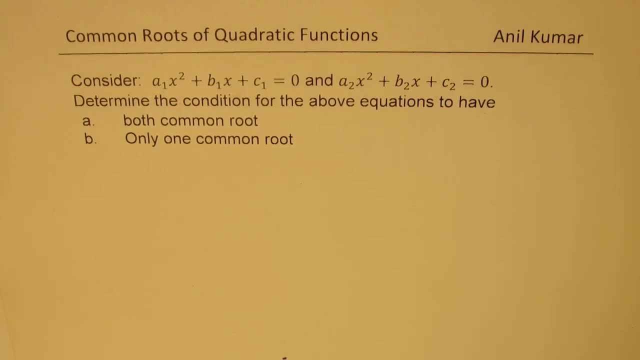 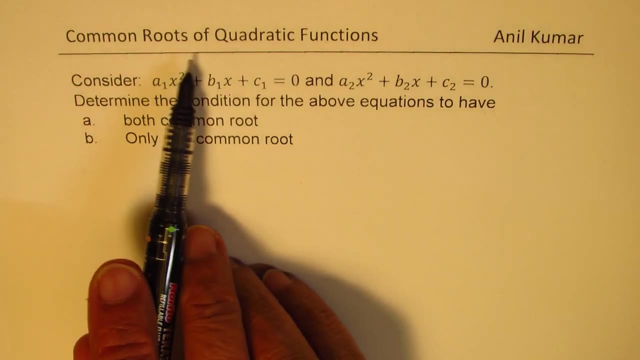 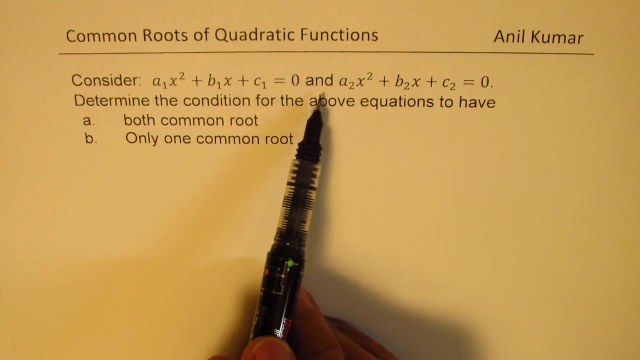 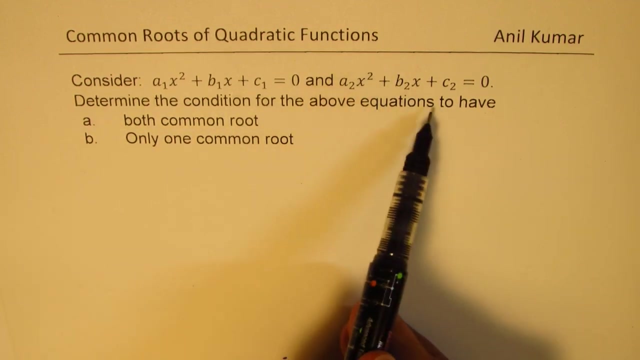 I am Anil Kumar. Welcome to my series on polynomials. Here we are going to take a very interesting question, and that is regarding common roots of quadratic functions. Consider: a1x square plus b1x plus c1 equals to 0, and a2x square plus b2x plus c2 equals to 0.. Determine the condition for the above equations to have both common roots: only one common root. So these are: 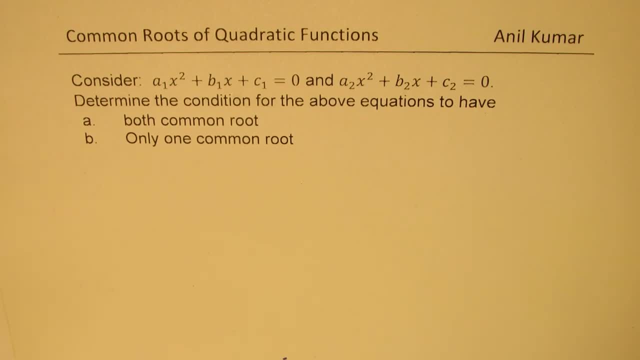 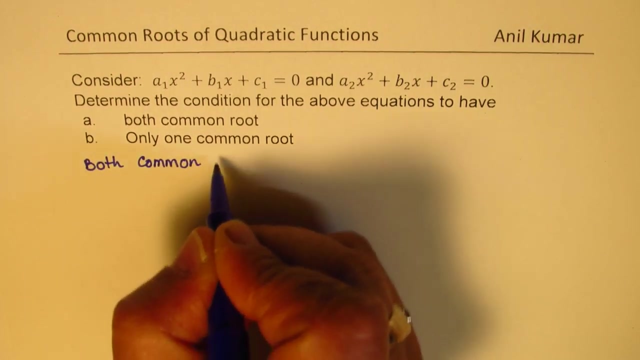 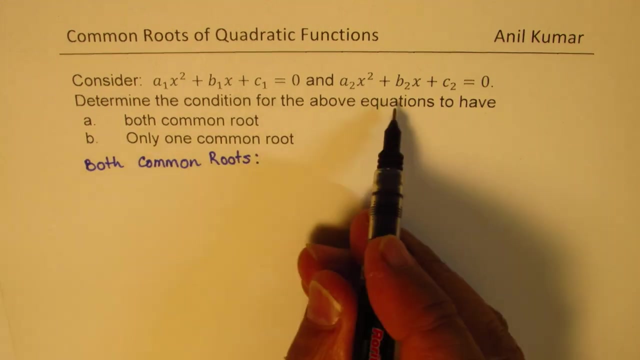 the two parts of the question which we are going to do. This is extremely important from test point of view, right? So let us first consider the case when we have both common roots. Now, that means both the equations have same roots, right? So let's say the roots are alpha and. 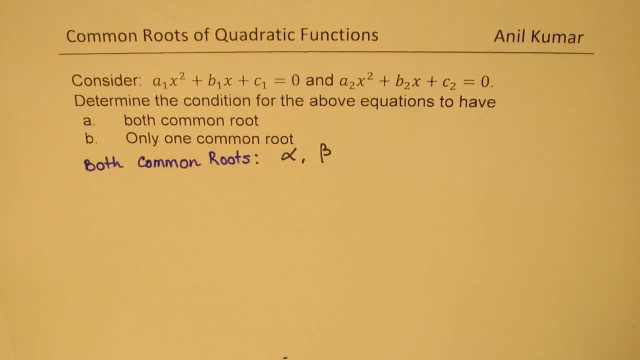 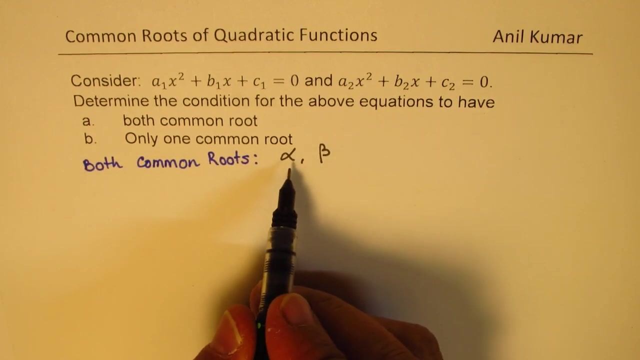 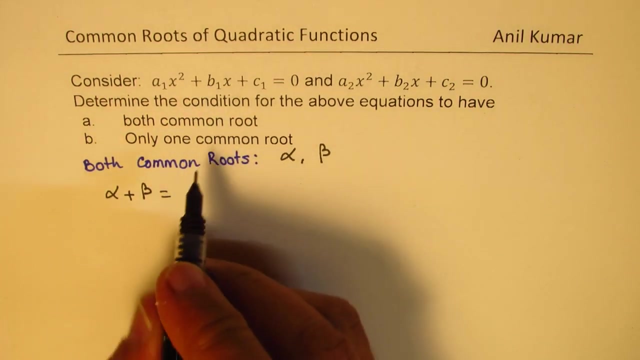 beta, right? So these are the two roots which are common to both of them. right Now, what does it really mean, right? If we have two roots as common? in that case, the equation should be: what? Then we know that, alpha plus beta, the sum of these two roots will be minus b over a right. 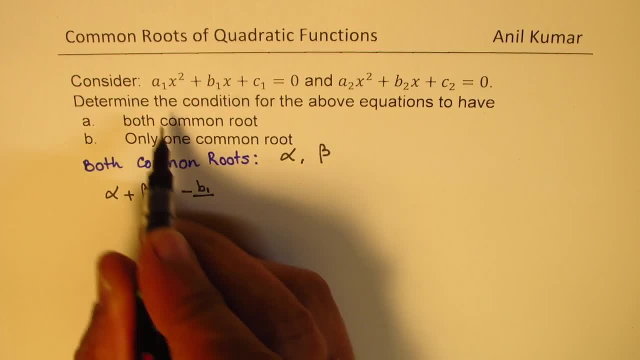 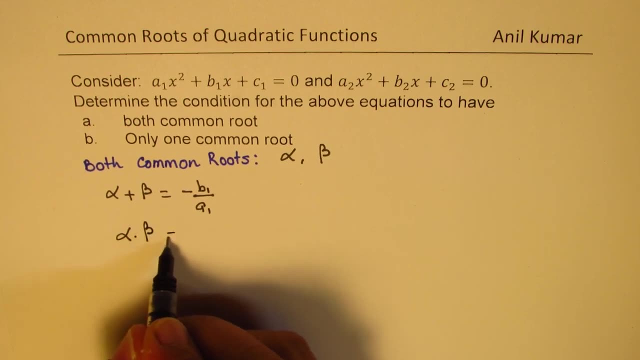 So in the first equation it will be B 1 over a 1 right, and the product of these two roots, alpha and beta, will be C: 1 over a 1. good, so this is from the first set of roots right now, since they. 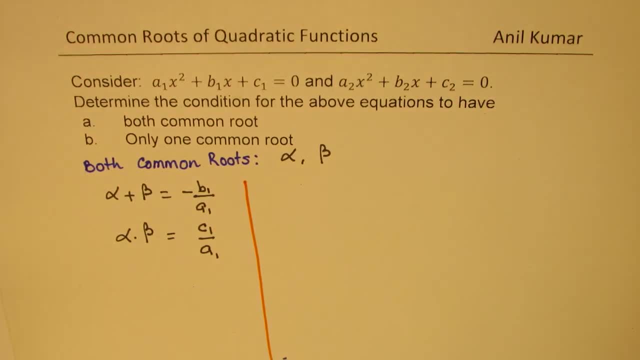 are common. right, since they are common, we also have from the second set of equation that alpha plus beta is equal to minus b2 over a 2, and alpha times beta equals 2 C 2 over a 2. is that clear to you, right? perfect now, from here we. 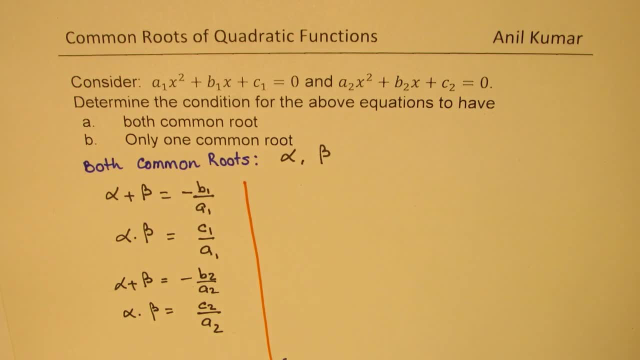 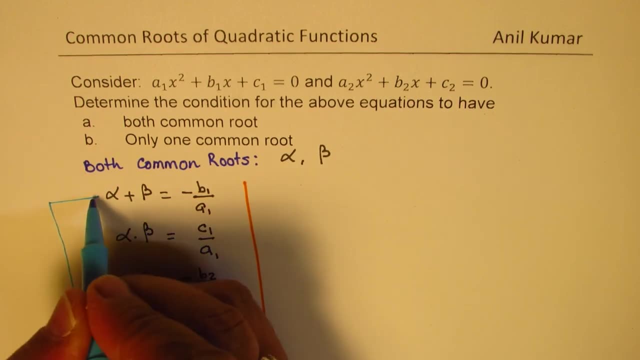 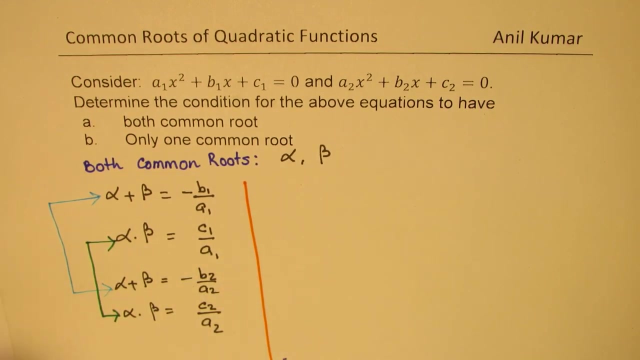 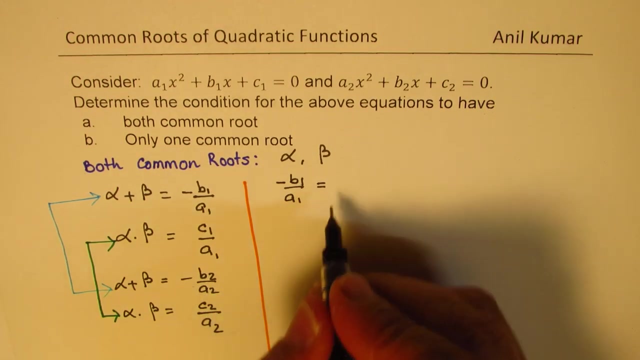 could relate very easily, right? so let's connect these, so the roots of com. then we have alpha plus beta. these should be equal, correct? And their product, they should also be equal, right. So it really means that I could write that minus b1 over a1 should be equal to minus b2 over a2, right, And that? 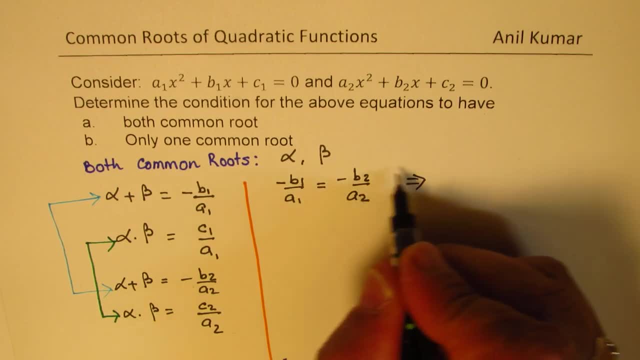 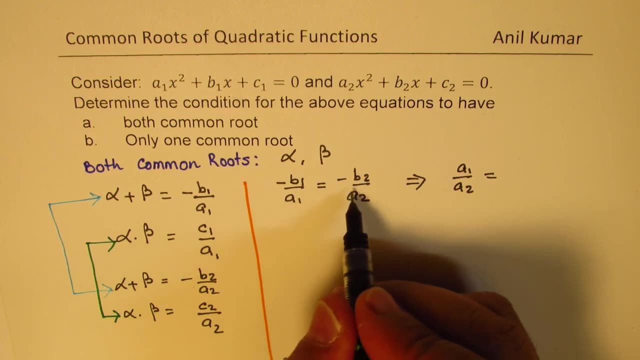 means what? This means that a1 over a2, we just cross, multiply, right, So we get a1 over a2 and is equal to b1 over b2.. Perfect, Okay, So this is what we get from our sum of roots. 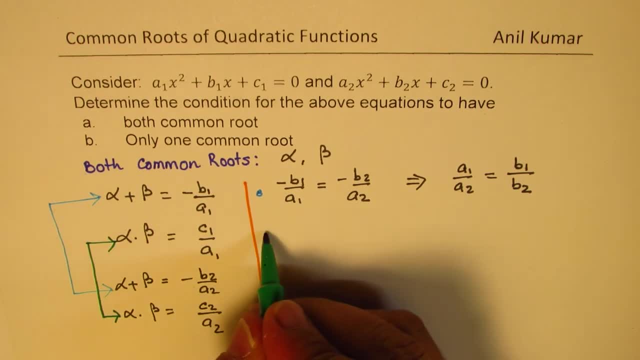 And now, if we compare the product of roots, what we get is that we get a1 over a2.. So we get a1 over a2.. So we get a1 over a2.. So we get a1 over a2.. What do we get? We get c1 over a1 equals to c2 over a2.. That implies that a1 over a2. 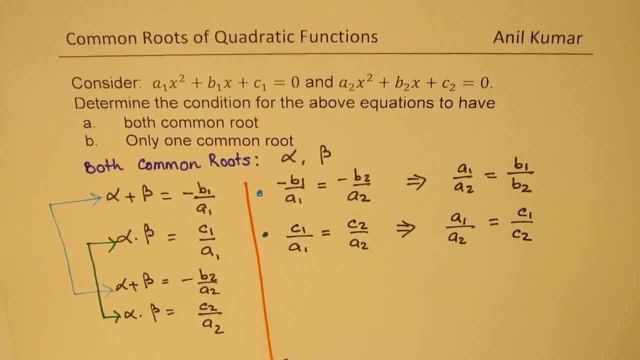 is equal to c1 over c2, right? So the condition is very clear to us: combining these two now, So you can combine these two correct, You should get what You get. a1 over a2 is equal to b1 over b2 is equal to c1 equals to c2.. That means these coefficients are in fixed ratio. 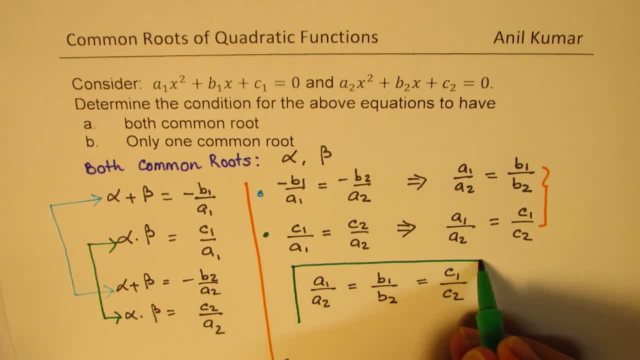 correct. So that is the condition for both the quadratic functions to have exactly same roots, right? So I hope you understand the situation. It is kind of what It is that we have a graph, maybe kind of like this, right The. 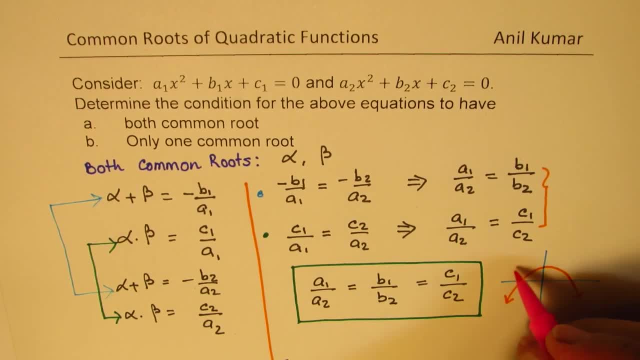 the other graph. they have the same roots means it could be something like this, right? So you see, there are common roots. It could be even like this: So that is what we mean when we say both common roots, correct? So if that is the case, in that case the ratios. 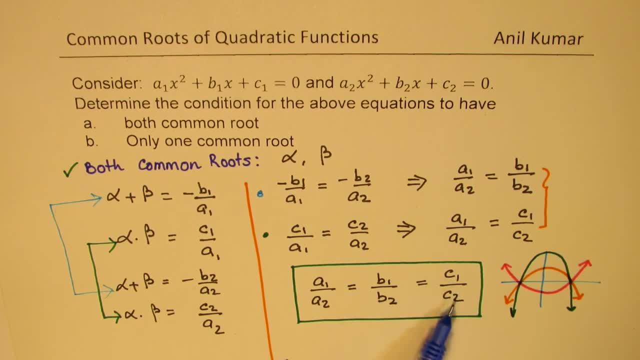 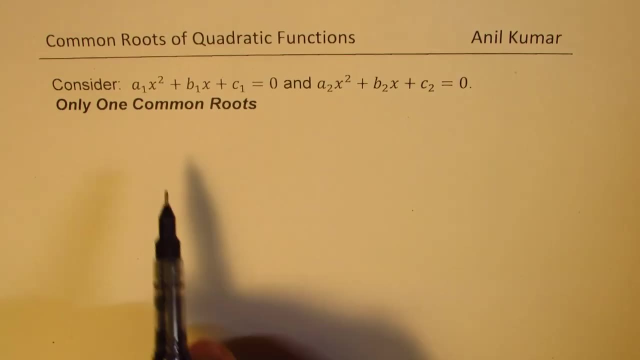 of their coefficients should be equal and the ratio of constant, that is the constant value. Is that clear to you, Right? So that is clear. Now let's get into part b, which is only one common root. perfect, So let's look into that now. Now let us take the second part. We'll consider the same two. 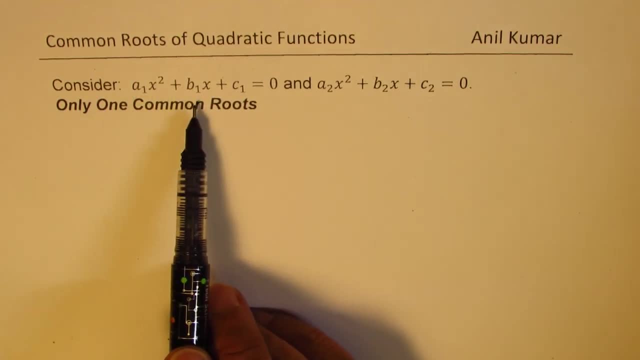 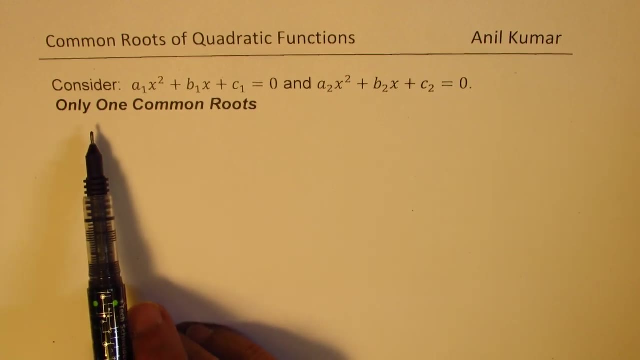 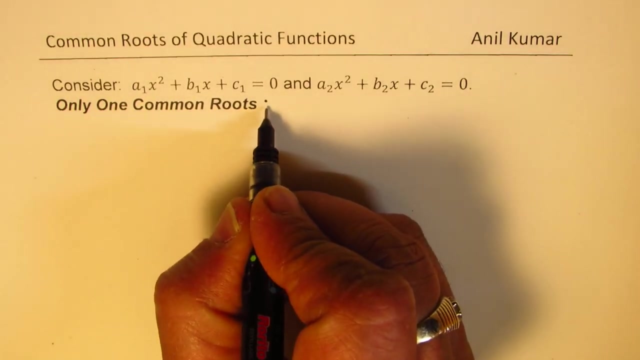 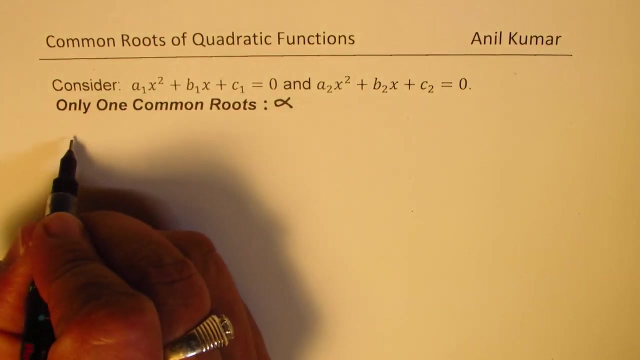 quadratic equations: a1 x square plus b1 x plus c1 equals to zero, and a2 x square plus b2 x plus c1 equals to zero. We're looking for the solution. when there is only one common root, Let this common root be. let us say alpha. right, If alpha is the root. in that case the equation could be: 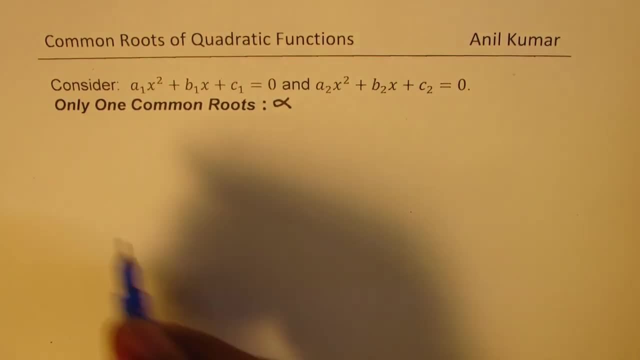 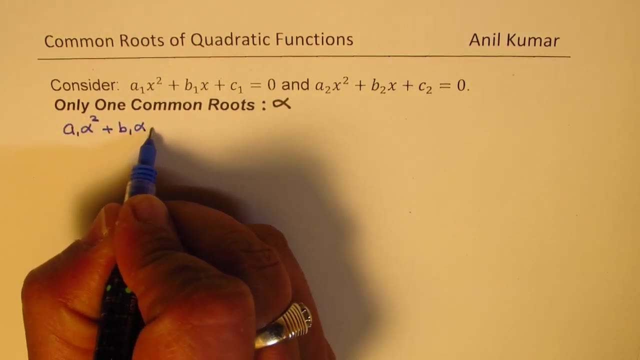 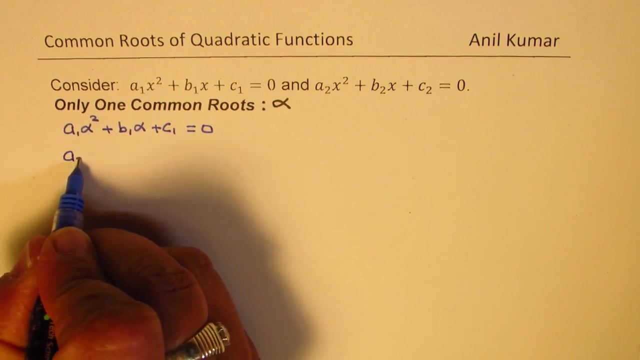 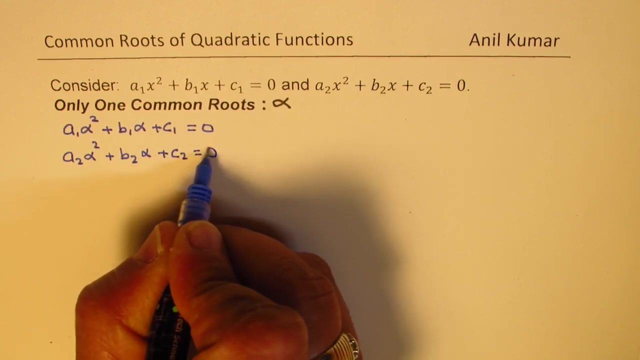 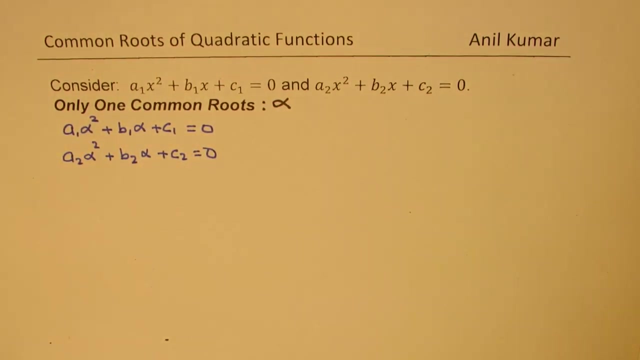 written as: a1. alpha square plus b1. alpha plus c1 equals to zero. and we could write the other equation as: a2 alpha square plus b2. alpha plus c2 equals to zero. right, Since alpha is the common root, if I substitute the value of alpha, I should get zero as the answer right for this particular. 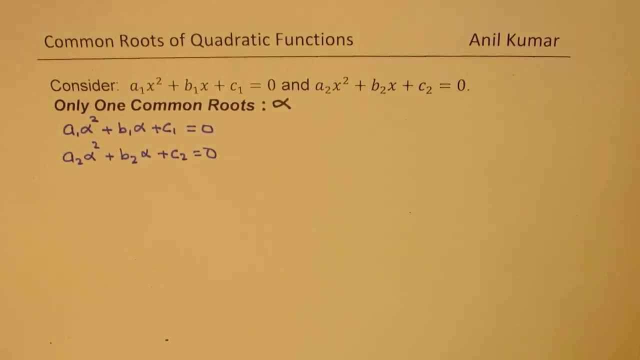 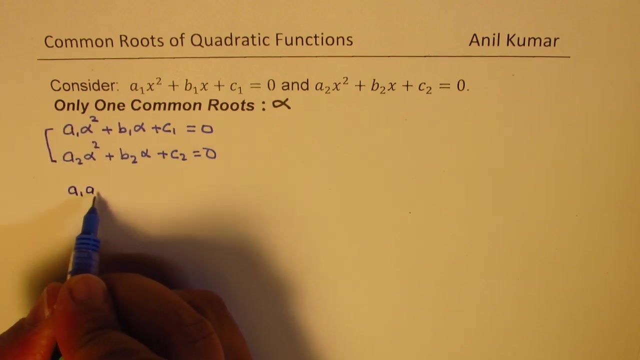 equation right. It should be satisfied with this value of alpha. Now, if I multiply the first equation by a2 and the second by a1, so it will consider these systems of equations right. We get what We get: a1, a2, alpha square. 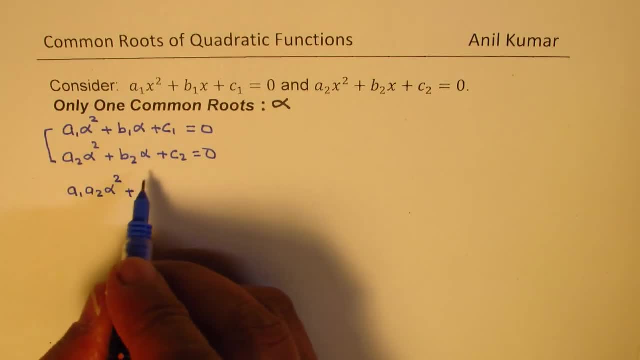 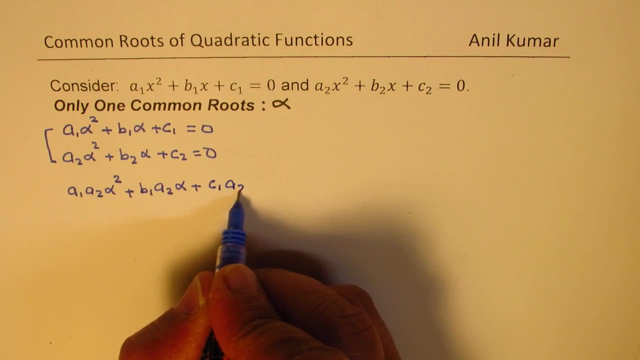 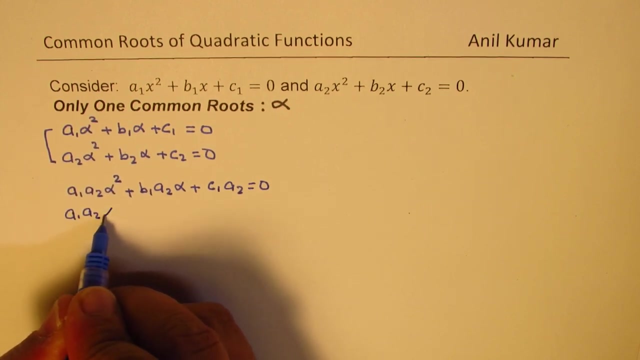 plus b1 a2 alpha plus c1- a2 equals to zero. and if I multiply this with a1, then I get a1- a2 alpha square plus a1- a2 alpha squared. Huh, Subject to the confrontationalısıfe neste Tool Ĺ dominin r. Subject to the confrontationalısıfe neste Tool: Ĺ: dominin r2. dominin r2ร. sudahml фplac quý instagramappäh Assamni apramowicz. Play with English, نه, Yes, if a2. My second question is: 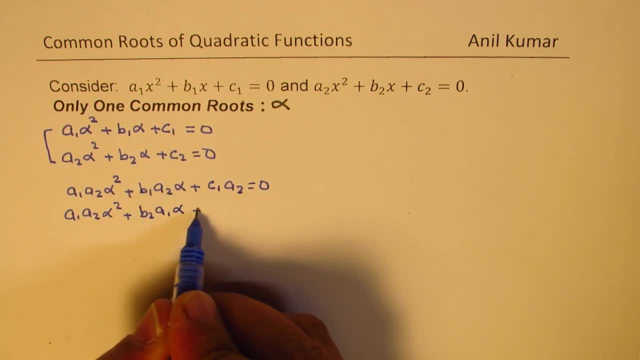 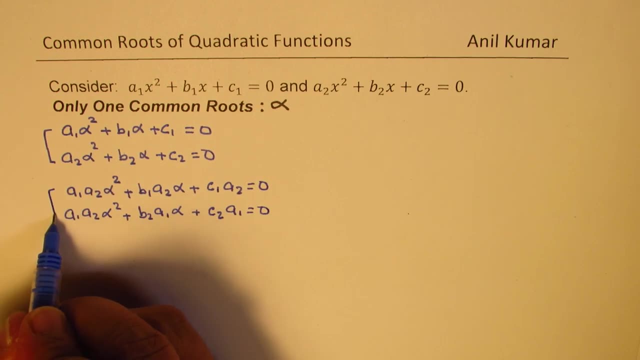 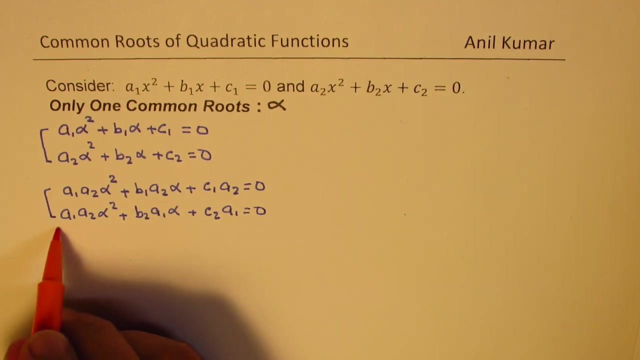 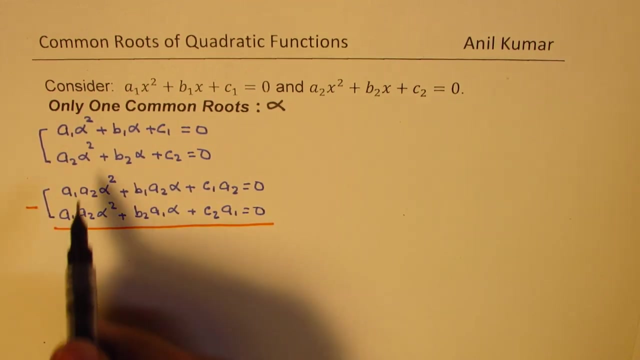 you can write: b2, a1, alpha plus c2 a1 equals to 0. Now we get this set. Now, if I take away one from the other, right, if I find the difference of these two, then see what do we get. So these two terms, they cancel and we get the value of alpha, right? so 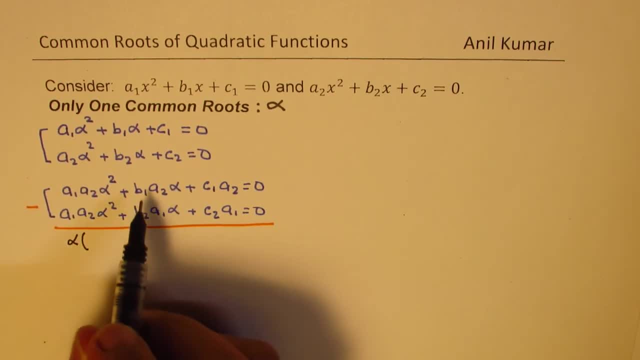 we can write this. alpha is common, so we can write alpha. and here we get b1 a2 minus b2 a1 plus c1 a1 minus b2 a1.. C 2, C 1, A 2 minus C 2 A, 1 equals to 0. ok, So that is what we get and from here we can. 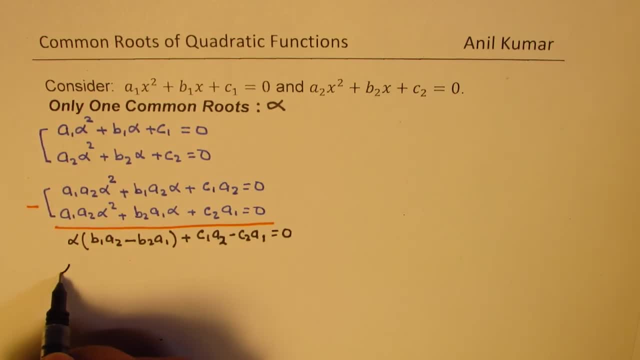 isolate alpha, taking this term to the next side. So we get alpha equals to now. if you take this, this becomes positive. So we get C 2 A 1 minus C 1 A 2 divided by these terms, right? So I write this as A 2 B 1, right? or we can write this as. either way we write this. 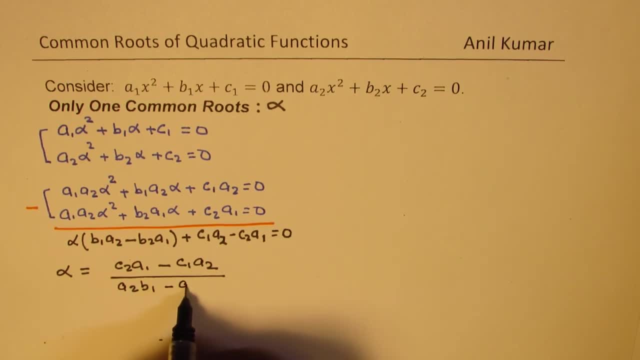 as A 2 B 1 minus A 1 B 2.. Right, you can actually also write this as A 2 C 1 minus A 1 C 2 over A 1 B 2 minus A 2 B 1, right? So if we change the order for both numerator and denominator, you could also. 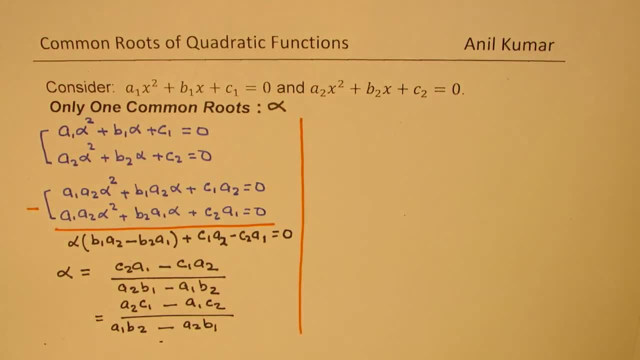 write this as shown here, Right, Ok, So that is how we could get the value of alpha. Now, if I multiply this equation by B 2 and the other one by B 1, then what happens? Now? what I am going to do here is: 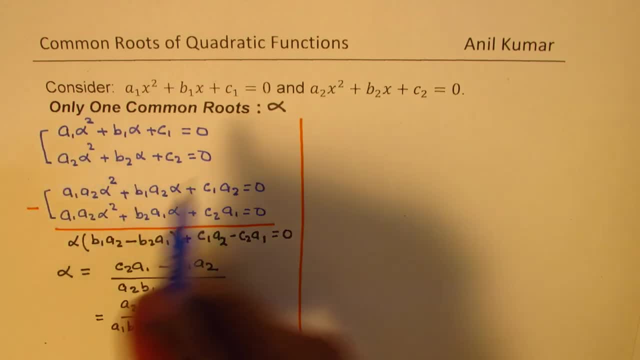 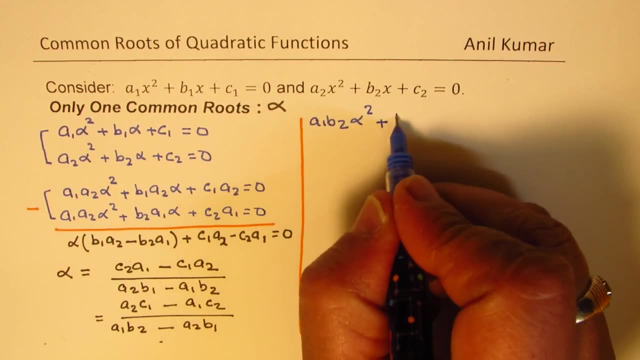 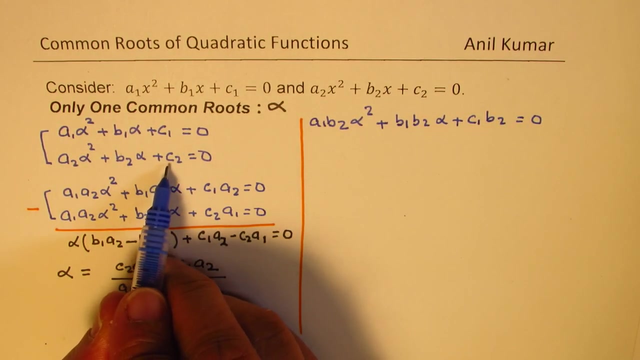 we are going to multiply this with B 1 and this by B 2.. So we get A 1, B 1, B 2 alpha square plus B 1, B 2 alpha, B 2 alpha plus C 1, B 2 equals to 0, and multiplying this one with B 1, we get A 2, B 1 alpha square. 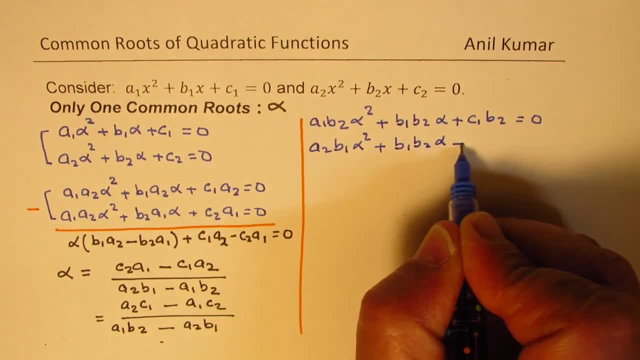 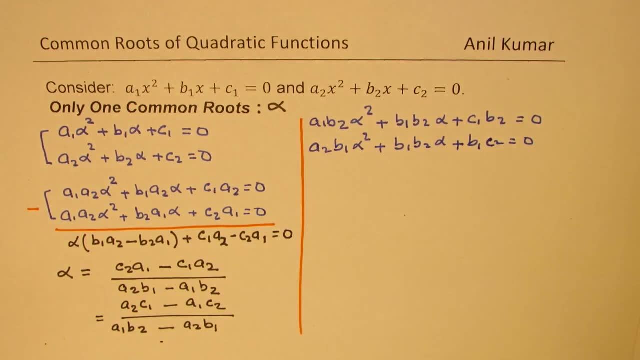 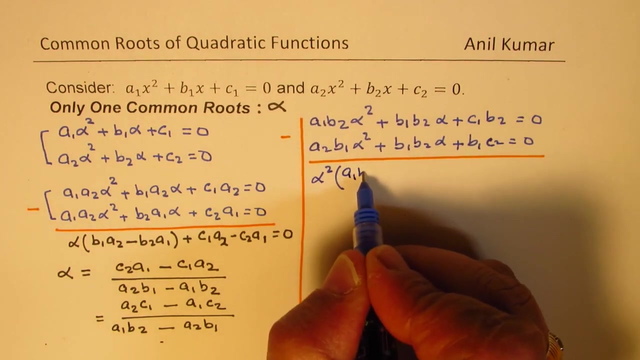 plus B 1 B 2. alpha plus B, B 1, C 1 C 2 equals to 0. right Now, if you take the difference now, if you take away these two equations, you get what Alpha square is right. So, subtracting, we get alpha square A 1 B 2 minus A 2, B 1.. These 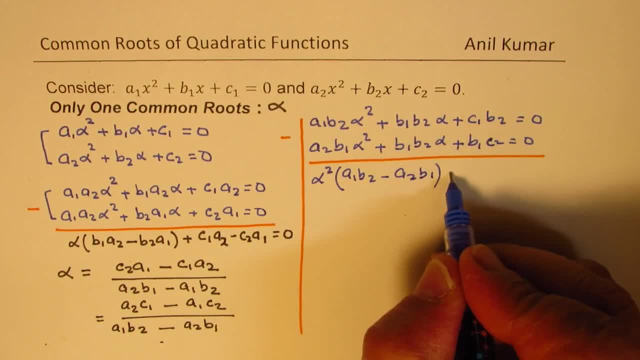 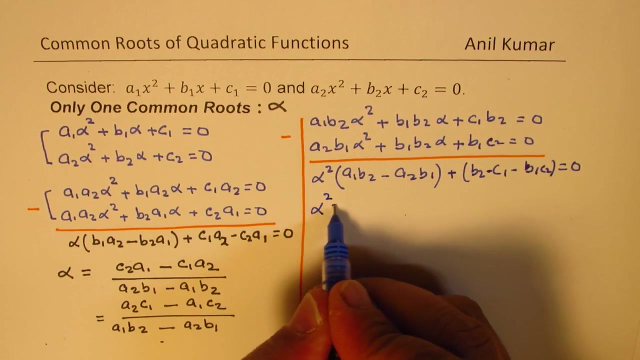 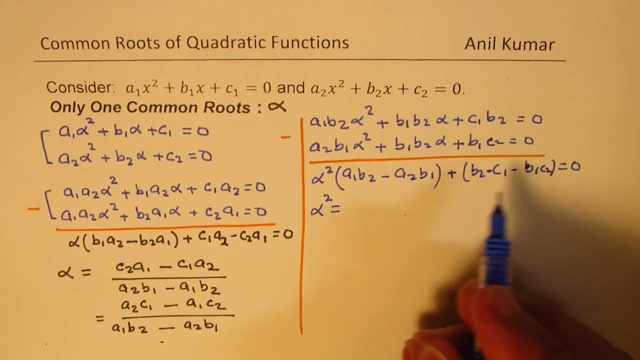 terms cancel, and here we get plus B 2- C 1, minus B 1 C 2 equals to 0, right. Or we get alpha square as equal to Right. So if we take this on the right side, in that case the order we can change and we can write. 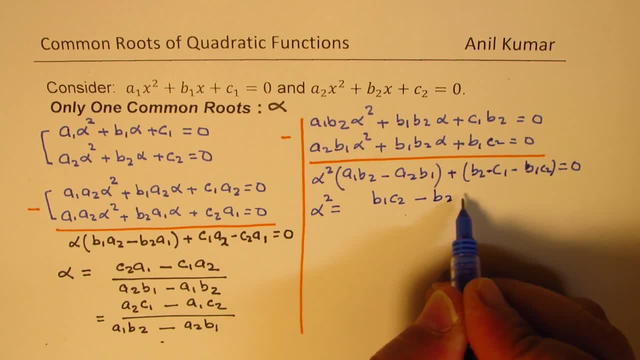 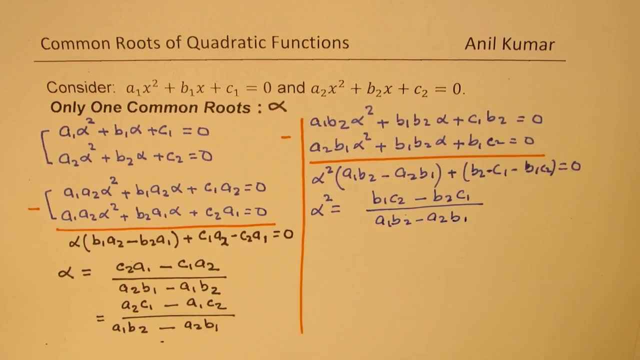 this as B 1 C 2 minus B 2 C 1, over this denominator, which is A 1 B 2 minus A 2 B 1, correct? So we get term for alpha square. This is alpha for us, right? Equation 1. let us say this is: 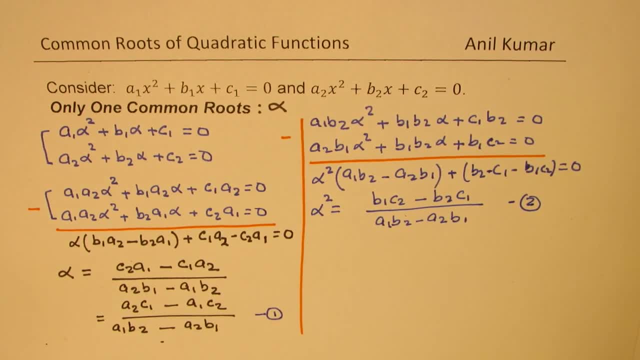 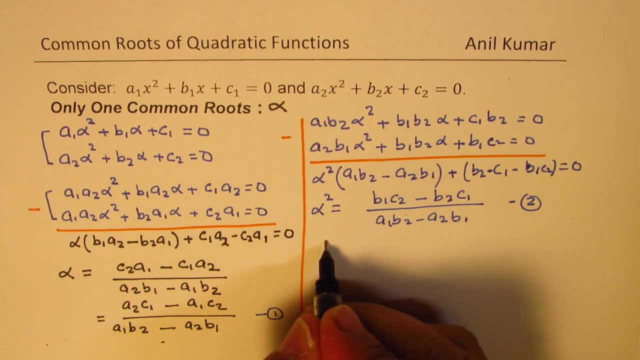 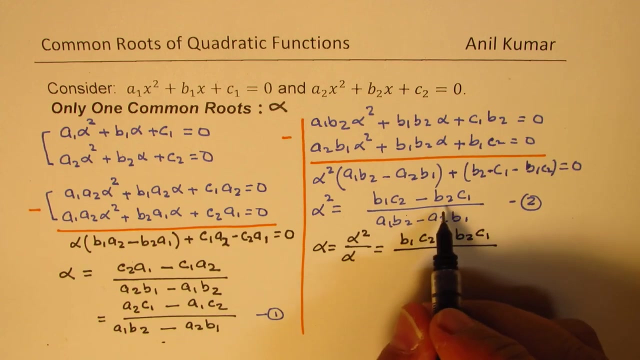 equation 2 for alpha square. 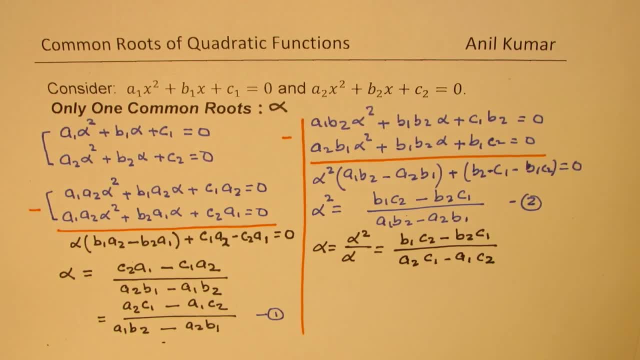 C 1 minus a 1 C 2, correct. so that is another expression which you get for alpha. and now we'll what we can see from here, that you know there are different ways in which we can find alpha. so this is another equation to find alpha, right? 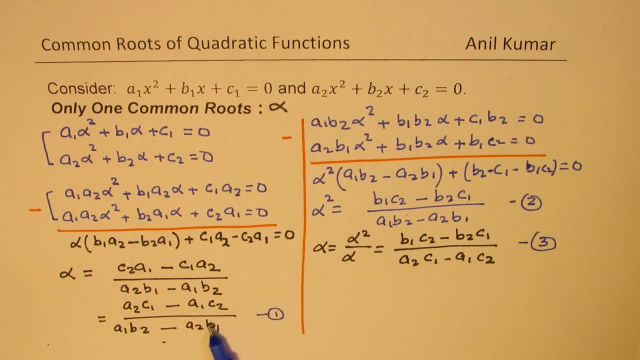 so you could either find using this formula or you could find using that formula, right, but anyway, both are alpha, so you could also equate them, and that is to say that we could also write from equation 1 and equation 3 that both are equal and therefore you can say that B 1 C 2 minus B 2 C 1 divided by all this, 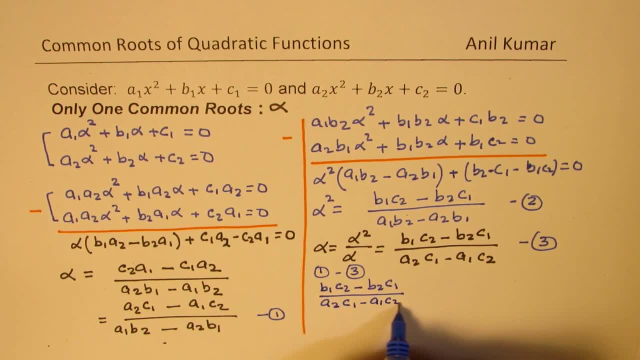 which is a 2 C 1 minus a 1 c 2, should be equal to this, which is a 2 C 1 minus a wholeelen of this kanji and fitting them together. so that is a 1 C 2 equal to 1 C 2. 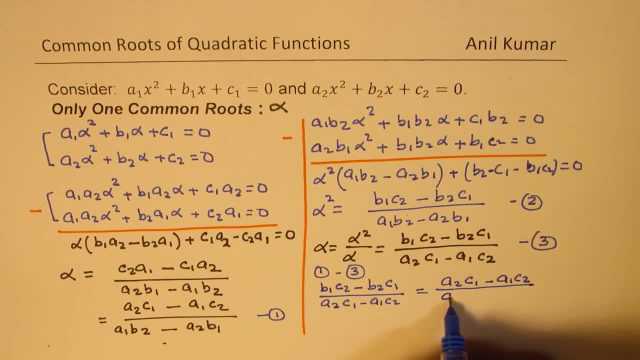 a1- c2 divided by a1 b2 minus a2 b1.. Correct. Now, if we cross multiply, then what do we get? So here we have a1, a2, c1 minus a1 c2, which is same as this right. 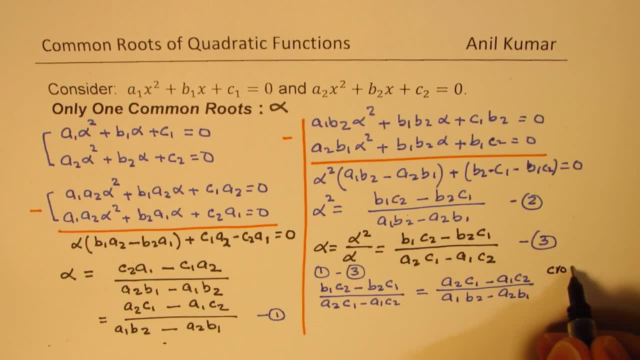 So if we cross multiply now, we'll cross multiply. So when we cross multiply, you get a1, b2 minus a2, b1 times this, which is b1, c2 minus b2, c1 equals 2.. The square of this, which is a2, c1 minus a1, c2, whole square. Now this is a very important formula. 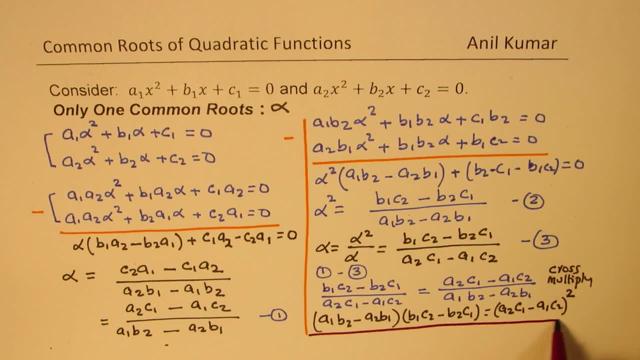 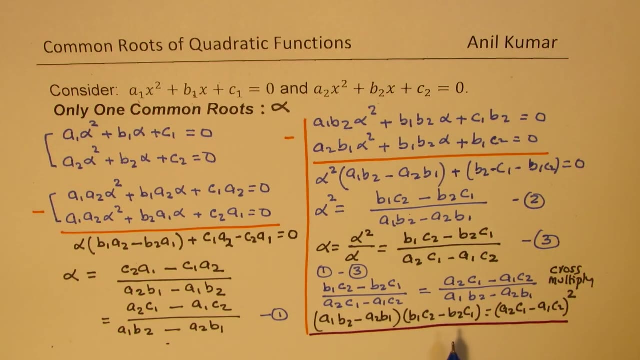 over here, Which you can remember, to solve questions based on only one root right. You also see that this product is a perfect square right, So that is another condition, So I hope that helps. Feel free to write your comments, share your views and, if you like, and subscribe to my. 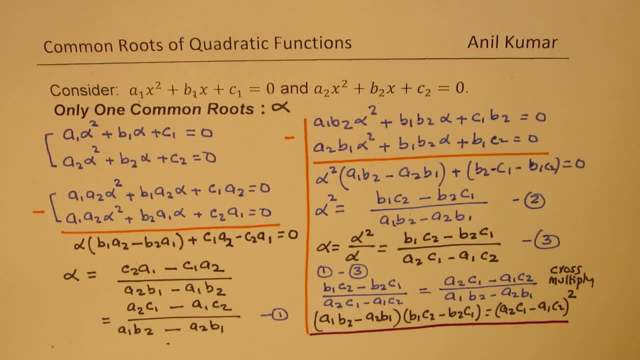 videos. that'd be great. Thanks for your time and all the best. 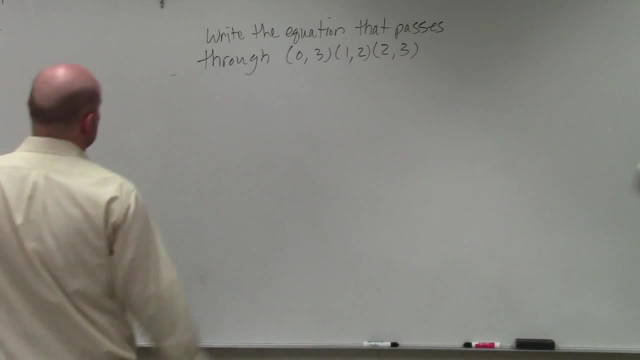 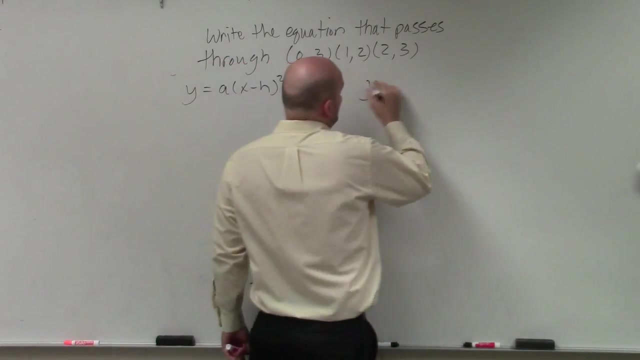 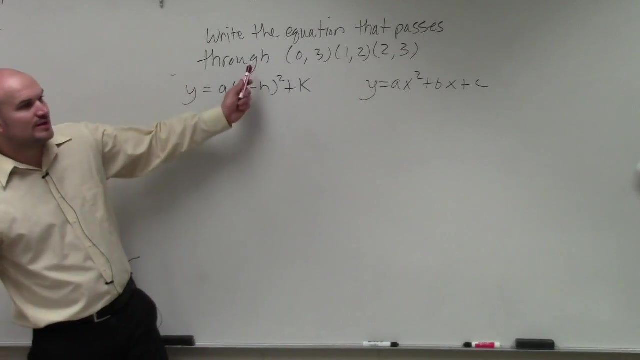 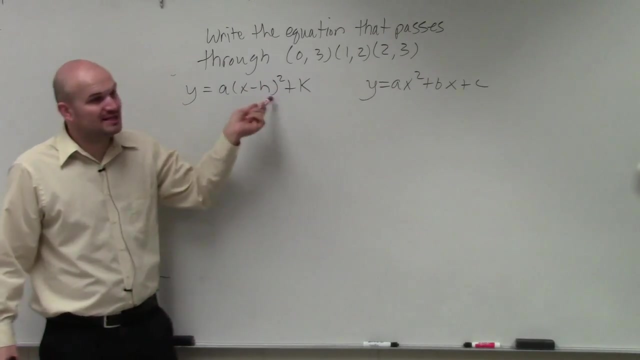 Again, as we talked about, we have: y equals a times x minus h squared plus k. vertex form. y equals a times x squared plus bx plus c, standard form. Now, do we know if any of these are the vertex? No, So guess what? This really isn't really going to help us that much, because